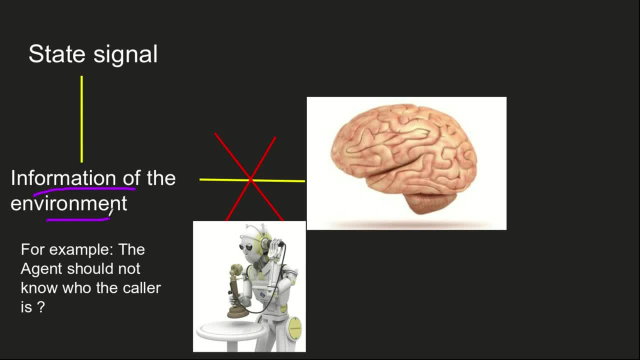 the phone, we should not expect it to know who the caller is in advance. Or, let's say, in a deck of cards. we don't want our agent to have information about the next card in the deck. In all of these cases, there is a hidden information in the environment and 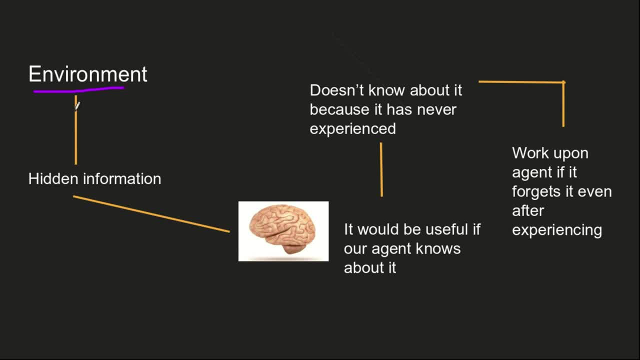 that information would be useful to us if the agent already knows about it. But the agent cannot acquire that information because it has never received or experienced such events. Briefly, we don't work upon our agent for not knowing something that matters, but only for having known something and then forgetting it. 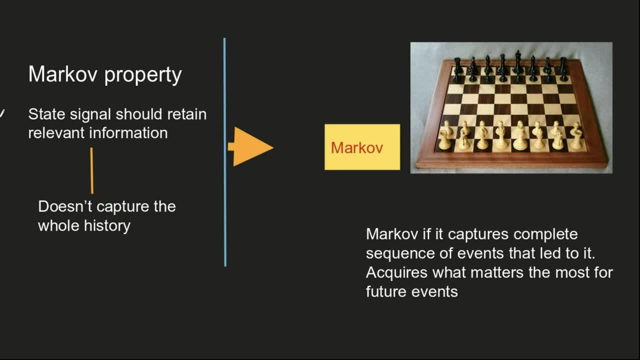 A State Signal summarizes past sensations compactly, In such a manner… that it retains all the relevant information. A state signal that succeeds in retaining all relevant information which is required for future is said to be Markov or to possess the Markov property, For example, let's say, our agent. 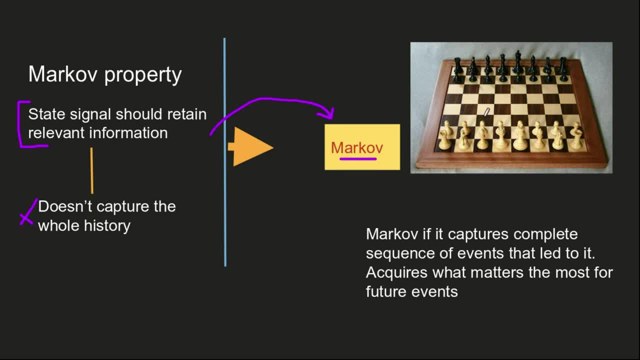 is dealing with different chessboard positions. The current configuration of all the pieces on the board would serve as a Markov state, because it will summarize everything about the sequence of positions that lead to it. Much of the information about the sequence of events that it has experienced would be lost. 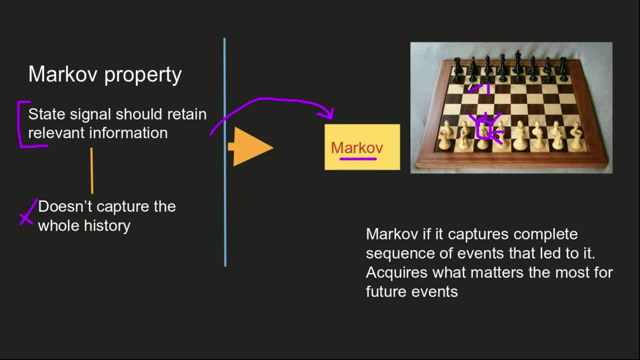 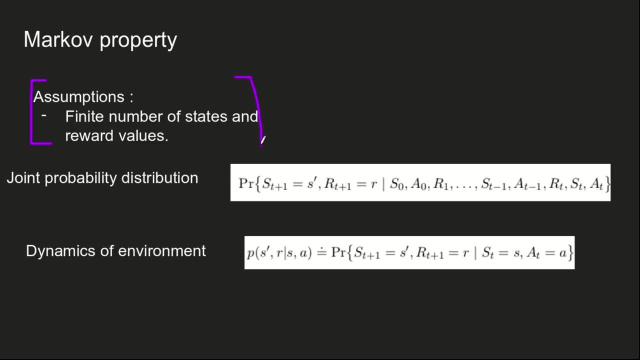 but all that matters is the future of the game, which is retained by the agent in the form of events. To keep the maths much simpler, we are going to assume here that there are finite number of states and reward through values. This enables us to work in terms of sums and probabilities rather than integrals, and 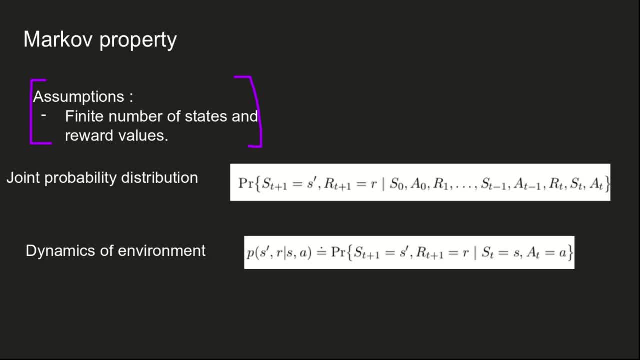 probability densities. Let's consider how a general environment might respond at a time t plus 1, to the action taken at time t. Dynamics of an environment can be defined only by specifying the complete joint probability distribution. So for all r, s and all these possible values of the 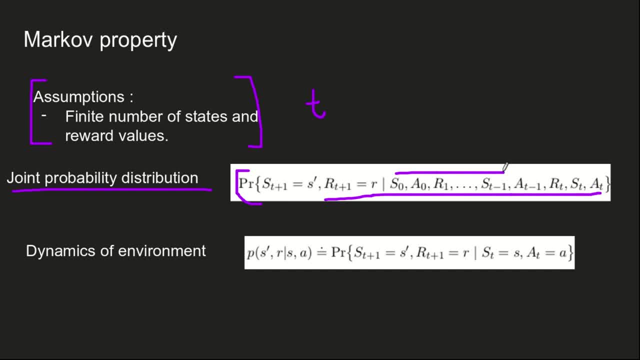 past events. s0,, a0, r1 to s, t-1,, a, t-1 denote past events. If the state signal has the Markov property, on the other hand, then the environment's response at t plus 1 depends only on the state and action's representations at t. So the 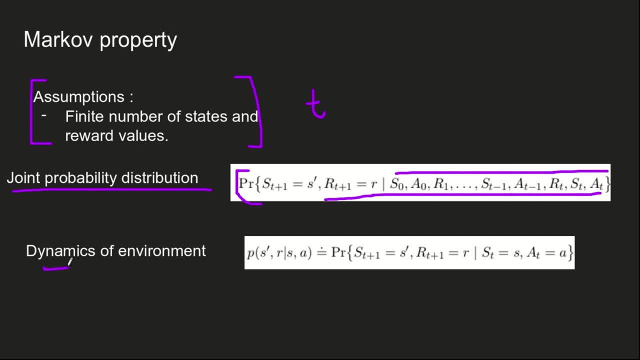 environment's dynamics can be defined by the following equation: for all r, s0,, s and a- In this case the environment and task as a whole are said to have the Markov property. If an environment is said to have the Markov property, then 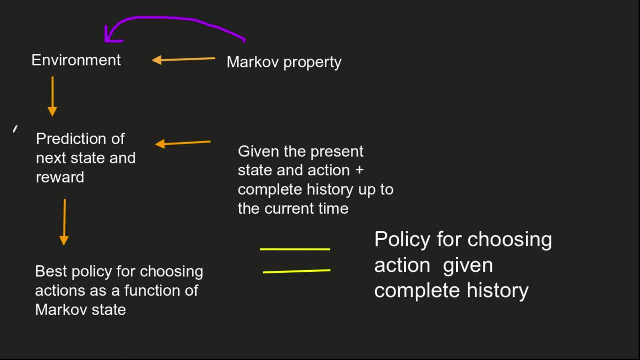 its one-step dynamics would enable us to predict the next state and expected next reward. given the current state and action, We can predict all future states and expected rewards from knowledge of the current state as well, as would have been possible given the complete history up to the current time. It also follows that 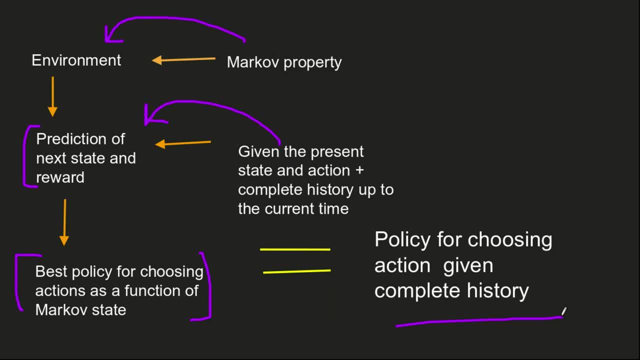 Markov states provide the agent with the best possible basis for choosing actions. That is the best policy for choosing actions as a function of a Markov state. The policy formed would be just as good as the best policy for choosing actions as a function of complete histories. 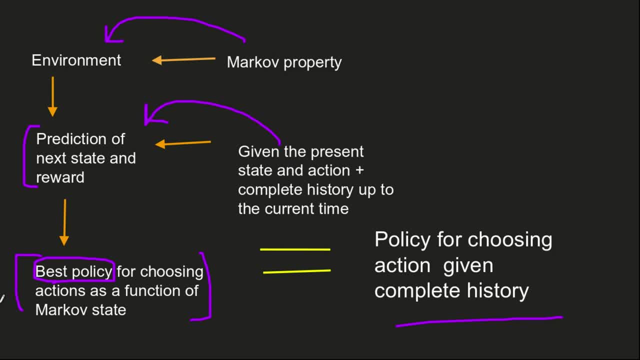 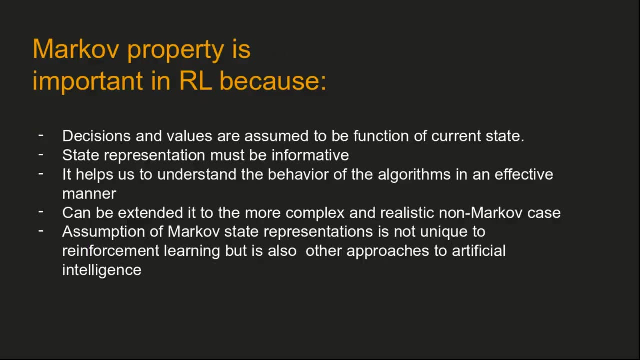 even when the state signal is non-Markov, it is still appropriate to think of the state in reinforcement learning as an approximation to a Markov state. In particular, we always want the state be a good basis for predicting future rewards and for selecting actions. Markov property is important in reinforcement learning because 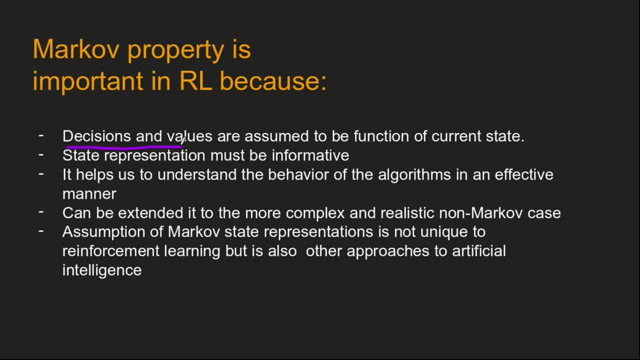 decisions and values are assumed to be a function only of the current state. so that they can be effective and informative, The representation must be informative enough. We usually assume Markov state signals. Markov state signals still help us to understand the behavior of the 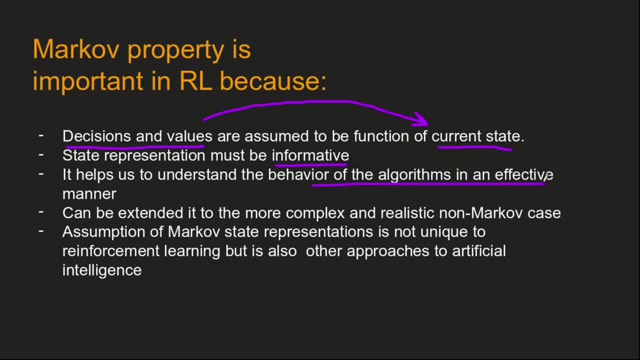 algorithms, and the algorithms can be successfully applied to many tasks with states that are strictly not Markov. A full understanding of the theory of the Markov case is essential foundation for extending it to the more complex and non-Markov case, which are realistic in some manner. 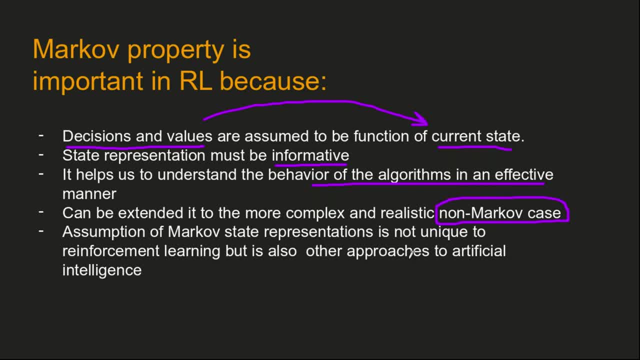 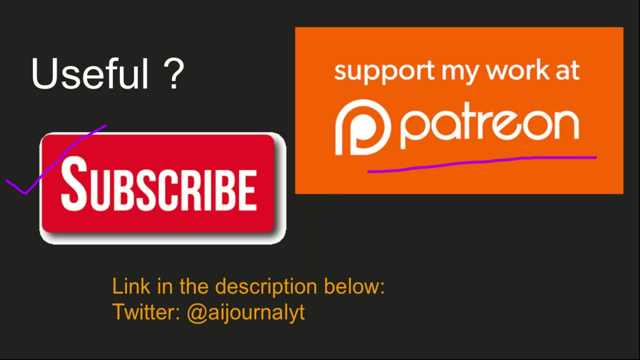 Markov state representations is not unique to reinforcement learning, but is also present in other approaches which are usually applied in deep learning and artificial intelligence. So with this we come to an end, and if you found this video to be useful, please subscribe to the channel and if you want to support our work, please support us on Patreon.